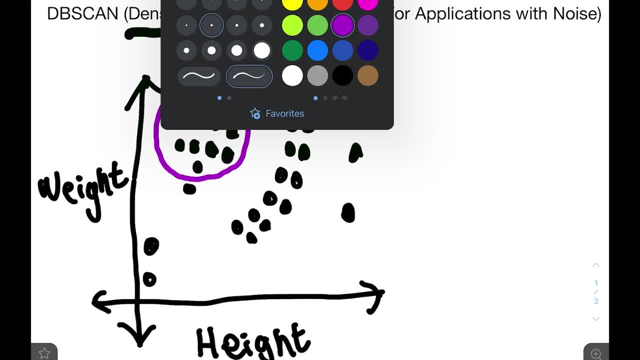 And then probably this other scoop actually should do a different color, a different color over here, specifying that this is a different cluster. So we'd hope that it identifies that we have one cluster in purple over here. We'll just call this number zero. 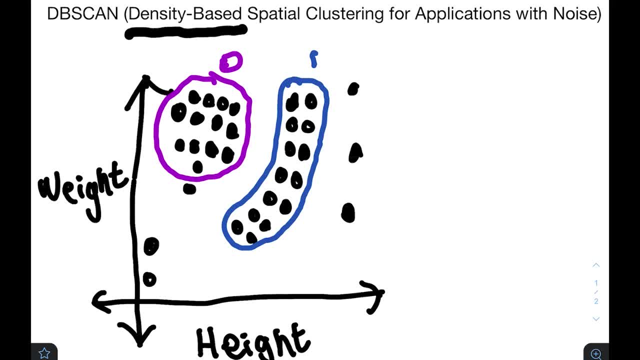 and that we had another one, which is cluster one over here, And then the rest of these- we kind of hope that it just calls them noise- And so we're going to specify that each of these are minus ones, because they're just outliers. 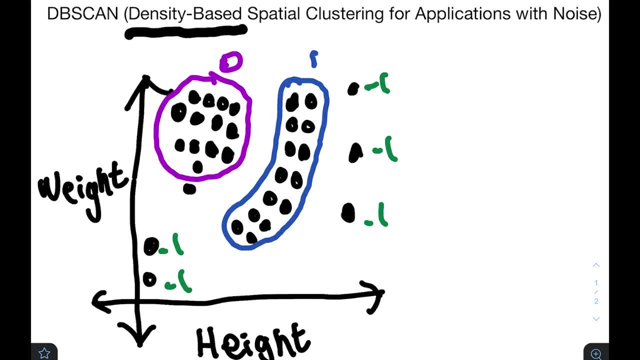 They really don't follow any sort of cluster. That's what we're going to hope happens, And if we do the DBSCAN algorithm, then it will actually output this or something extremely close. If we did the k-means algorithm- whether you know how that works or not- 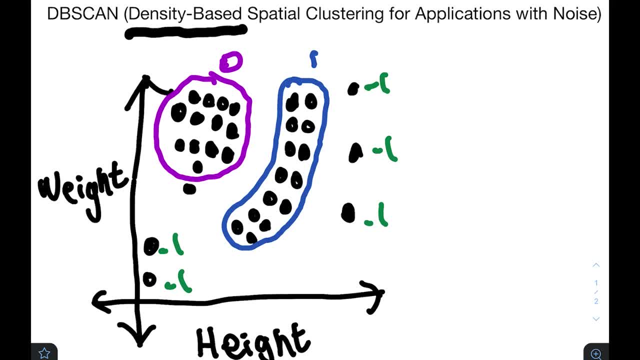 it would actually not get the right answer. most likely, DBSCAN is great with this kind of thing and we'll see what it does right now. So basically, how this works is we have to tell DBSCAN a couple of different things. We have to tell it epsilon. 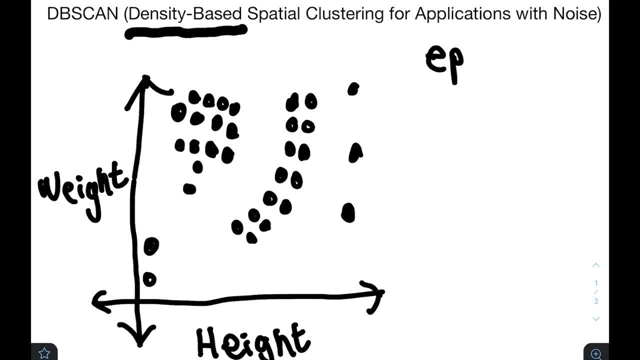 which is a distance value. We have to set epsilon, which I'll call eps, because that's what scikit-learn uses, And we'll set this equal to- for now, we'll say- 0.5.. And we also have to specify this thing called min-samples. 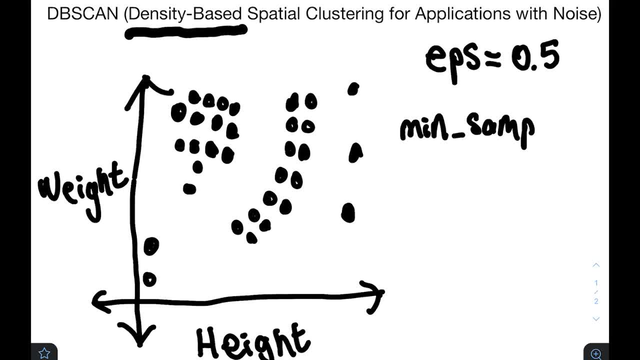 min underscore samples, And we'll set this equal to, say, 3.. Okay, so, when you're actually trying to find these correct values, well, there's a way of optimizing and fitting that, which I'll show you in the coding video if you want to see that. 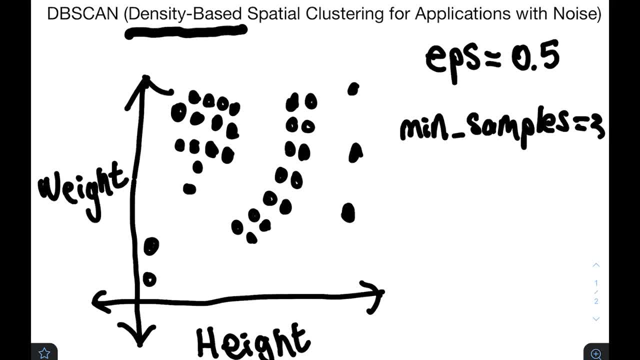 But for now we're just going to assume that we have some fixed values that you've decided. Epsilon is 0.5, and min-samples is 3.. Now what this epsilon value does is that epsilon equals 0.5. 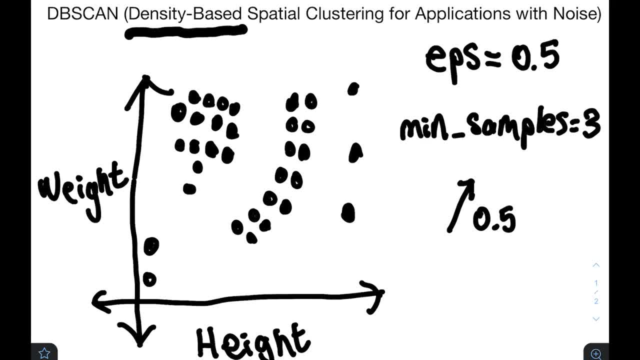 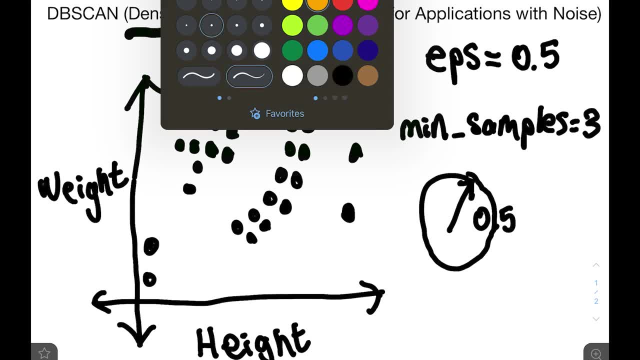 implies that the radius of a circle is 0.5. And so we could draw like a whole circle around like that- I know not perfect, but something like that- If we drew that circle around every individual point. well, we'll start with this one here. 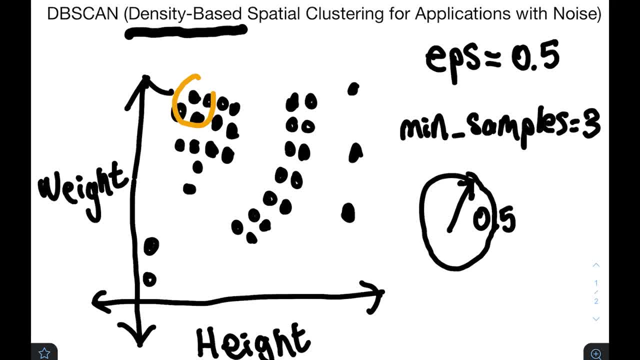 So we'll draw that circle and maybe it looks something like this And what it happens to do is hit three other points. Hey, sorry for this piece. I realize I need to explain this better. When I say the word hit, I don't necessarily mean. 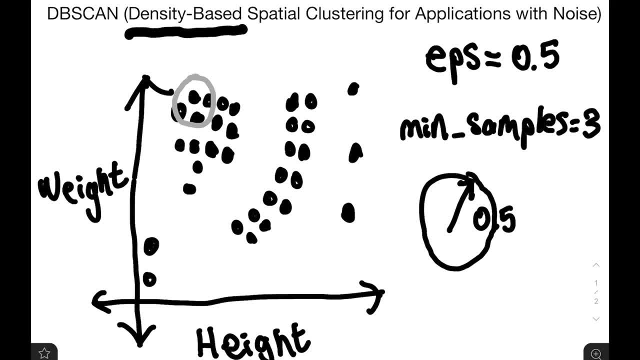 that the circle actually hits, as in absolutely touches another point. I mean that if the circle absorbs another point, So as long as there is other points that are within that circle, either on the boundary of it or anywhere within that circle, then that's what I mean by hit. 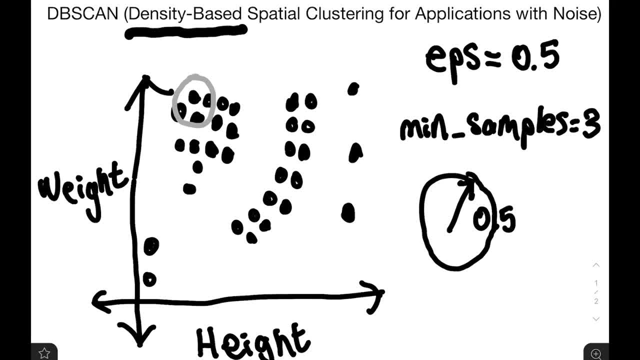 And if I say that carrying on forward, then that's what I mean as well. Anything within that circle, Carry on. It. hit this point, this point and this other point. If it hit three points, well, we'll just calculate that for now. 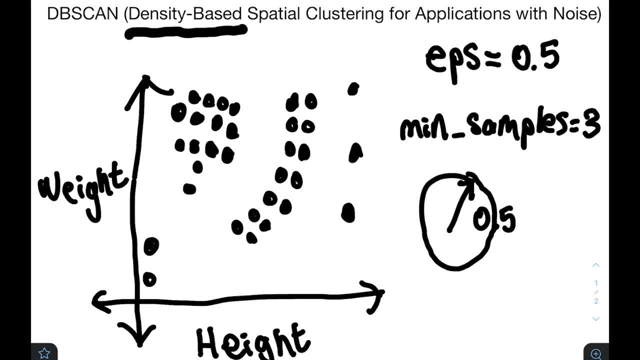 and remember that, that first point, that hit three with that circle. Now this second point, we'll do it for that That circle. if we draw it again happens to hit four other points and we'll remember that If we do that same process for every individual point. 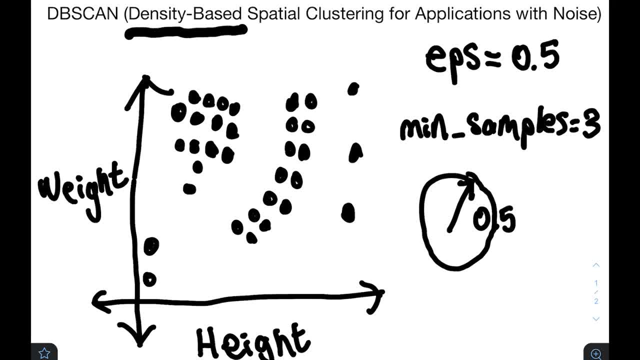 we will have memorized, and we can store that in the computer, how many different points that epsilon of 0.5 circle touches. So if we have that information, we have a whole number associated with each individual point And what we can do with that is compare it to this min samples value. 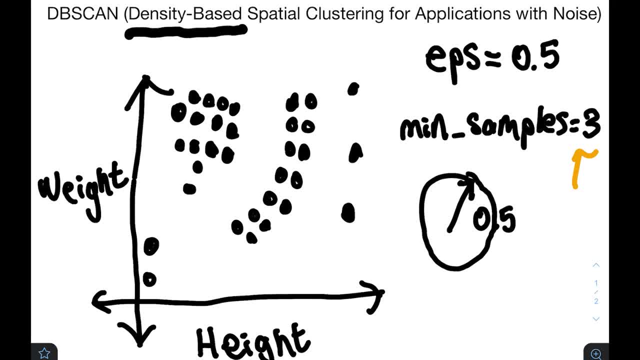 which is basically a threshold. If that threshold is set at three, then what we'll say is that if each point hits at least three different other points, it is considered what is called a core point. So many core points will be defined here. 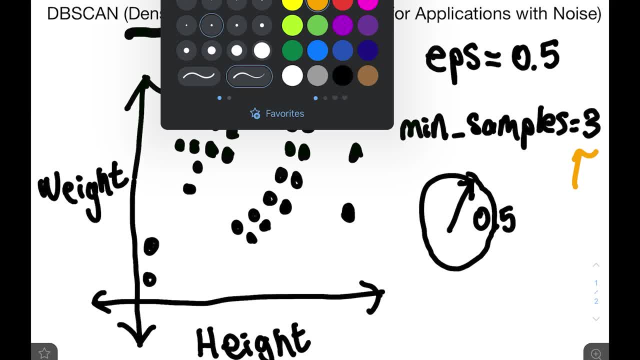 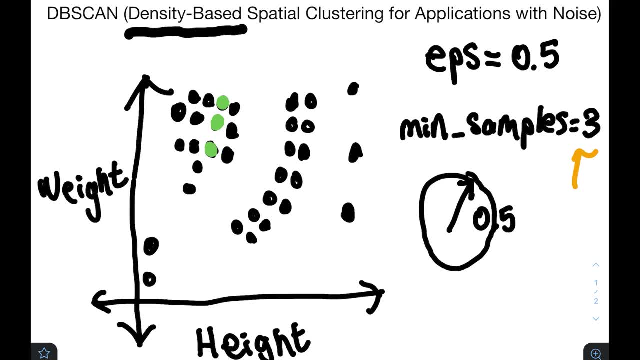 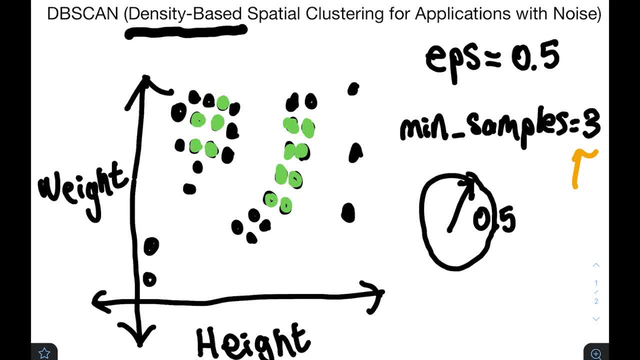 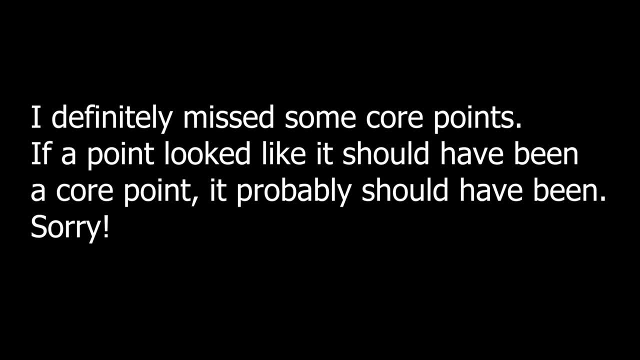 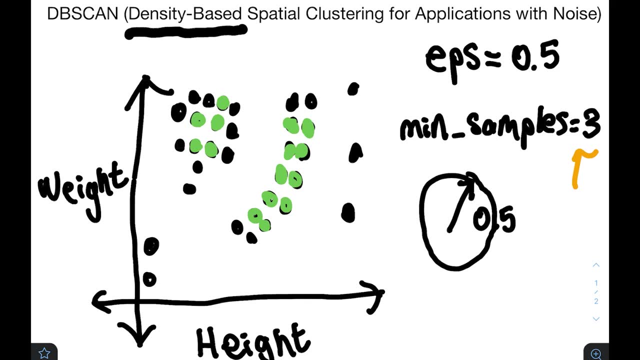 this is a core point, all of these other ones as well, And I'll just circle all of the ones that are most likely core points. Now that we've specified whether each point is a core point or not, we can do another process. 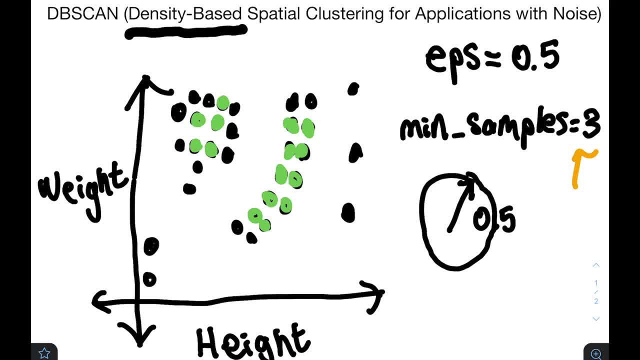 which is draw that circle again around each of the core points. So for each of those core points we will draw a circle around them. We'll start with say this one over here: If we draw that circle, it hits these points. 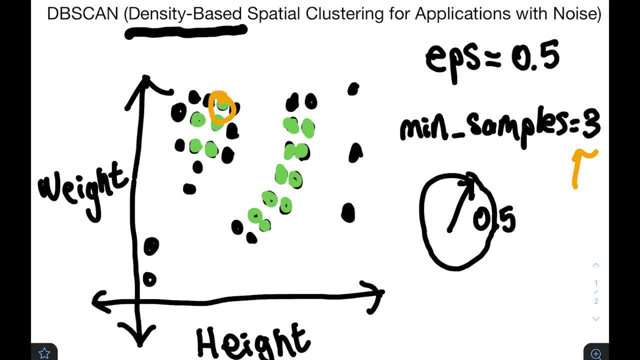 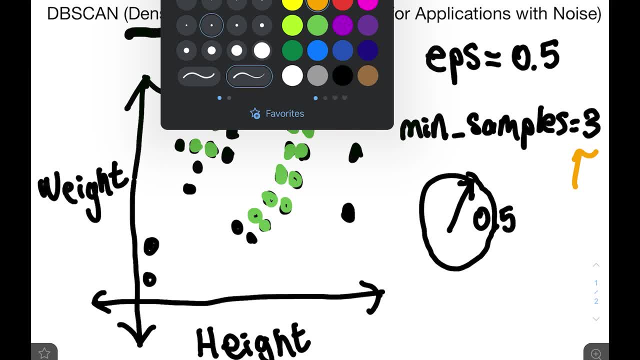 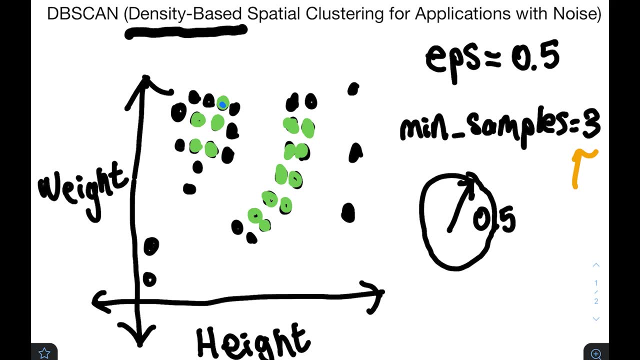 And now we are going to start specifying actual clusters, Starting one in not green, because this green is not specifying a cluster, it is specifying whether something is a core point. we will start in blue And, looking at this core point here, we'll start randomly with that one. 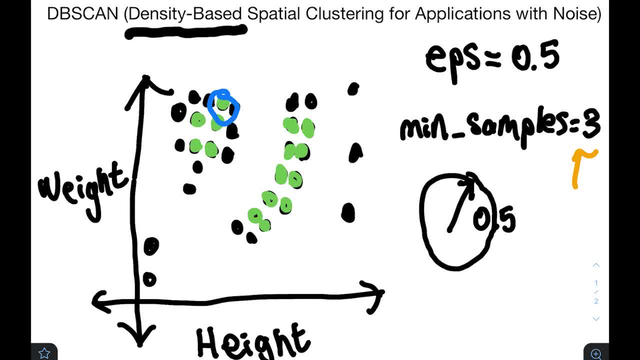 If we draw our circle, it hits all of these points, And so we will specify that this point is that cluster and all of the other ones that it touches. Now, for all of the other core points that it touches, we're actually going to draw that circle around them. 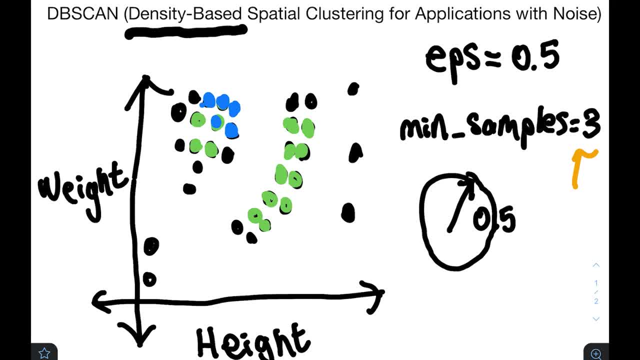 And so, since this is a core point right here, we'll draw that circle and then for each core point that it touches, we'll assume that those are part of that cluster as well, And we'll do that same process Now for the ones where it hits non-core points. 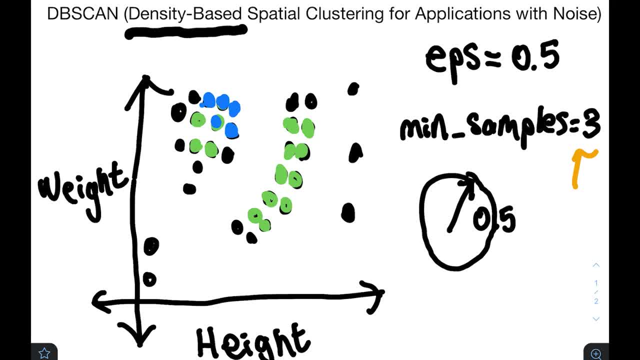 since that circle hit these non-core points, we are going to specify that these are part of the cluster, except we're not going to chain, react and bounce off of them and draw the circle off of these ones. We won't be drawing a circle like this. 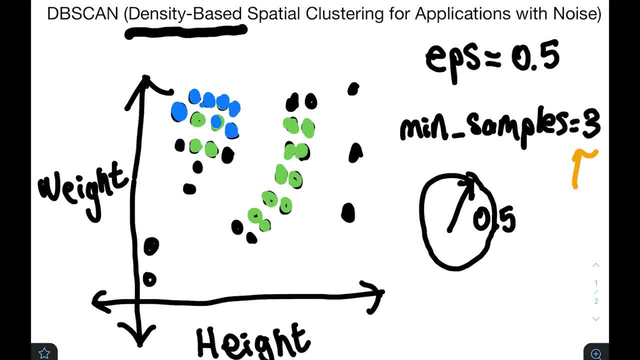 and seeing what they're touching. we're just going to classify them as those points. Now what should happen if you bounce around and do that chain reaction? every time we touch a core point, we'll bounce off of it and collect everything around it. 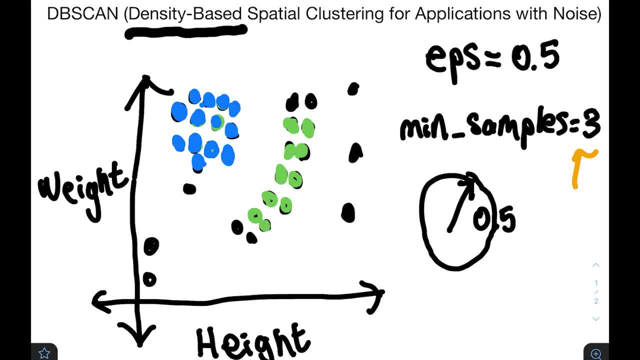 we should get something like this, Where all of these are assigned to that cluster and then this one here, since it's only close to this non-core point here and we don't branch off it, we don't chain react off of that. 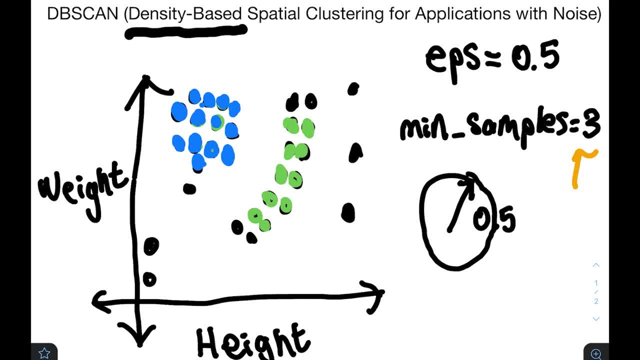 that point is not going to be specified as that cluster. This cluster is now fully done, identified and we'll just draw a zero to represent this is cluster 1, we need to identify more clusters because we have more core points. so for a random core point, 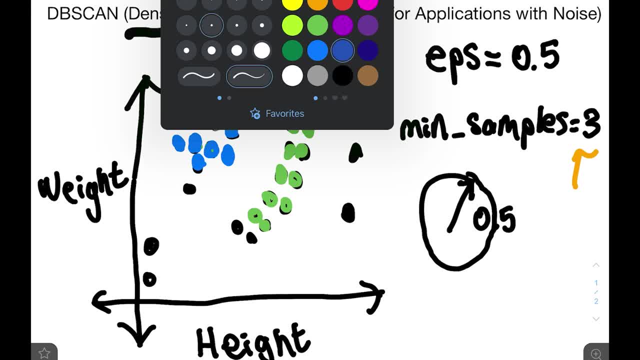 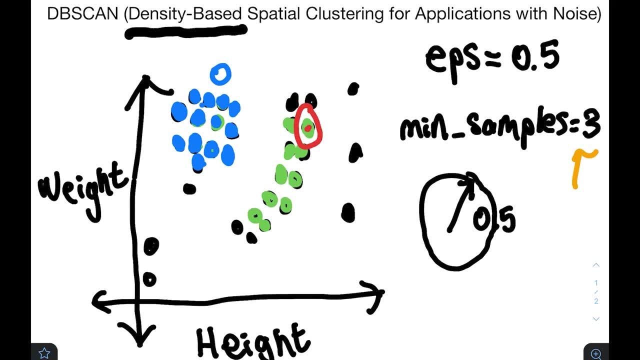 we start at one of those and start creating a new cluster. so we'll start calling this the red cluster and since this is a core point here, we'll draw a circle around it- maybe it hits these points- and we'll color each of those as a red cluster.